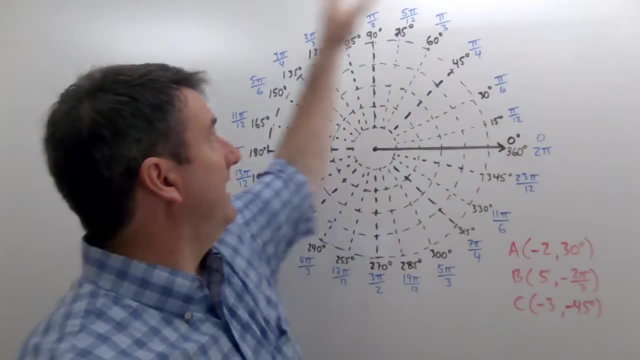 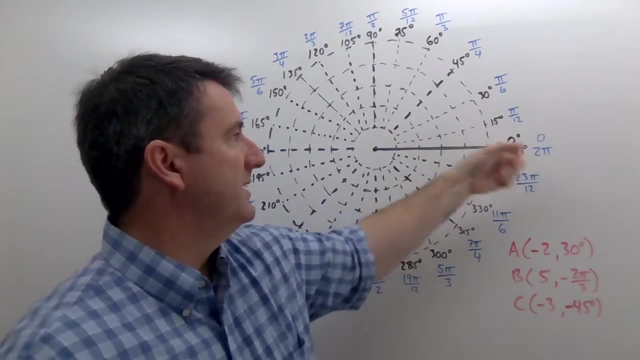 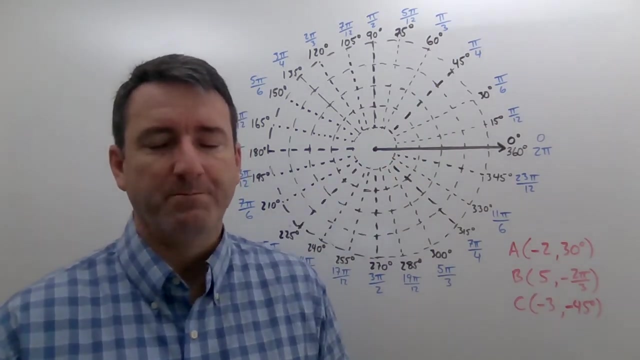 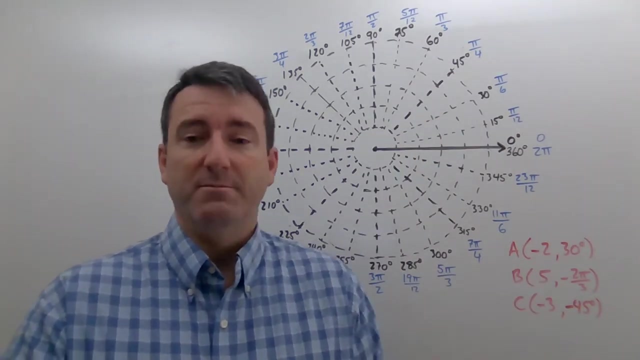 Our angle. we can give any direction by giving an angle between 0 and 360 degrees or between 0 and 2 pi radians, And we can give any distance as a positive value. However, when we start using polar coordinates, when we start doing some math with them, 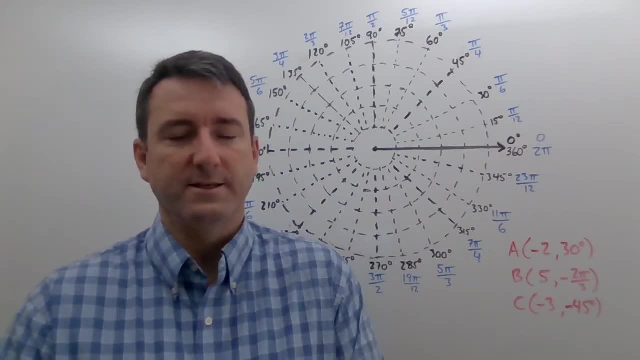 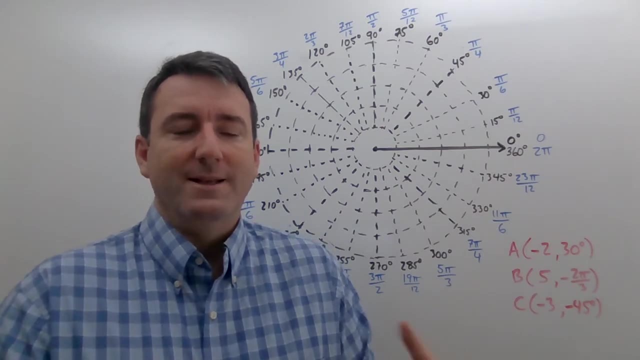 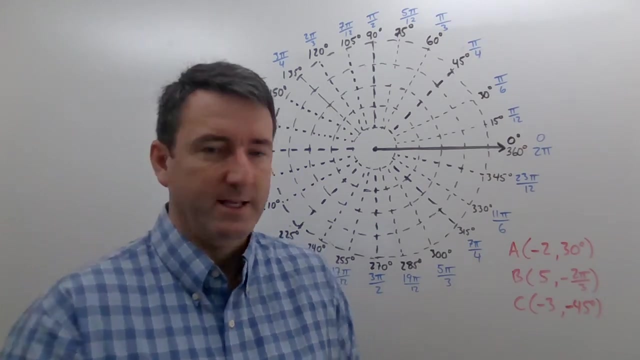 and especially when we get into polar equations and things like that, it's going to become necessary for us to we're going to come across some negative numbers in our polar coordinates And we so we need to think about what those mean. So what does it mean to have a negative angle? 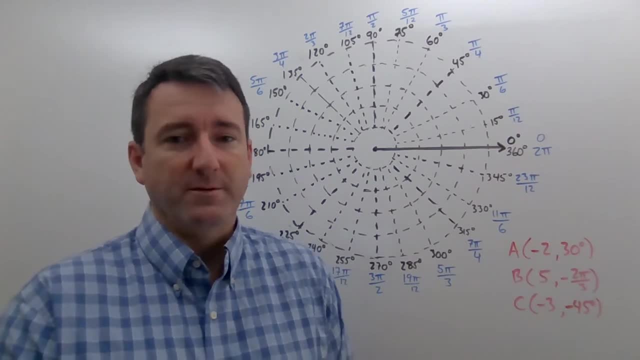 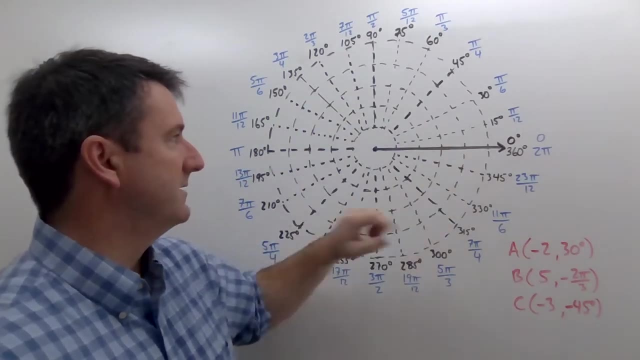 First of all, I'll start with angles, because we've already talked about those. Remember, in trigonometry we said that positive angles are measured in the counterclockwise direction And if we measure in the clockwise direction, that's a negative angle. 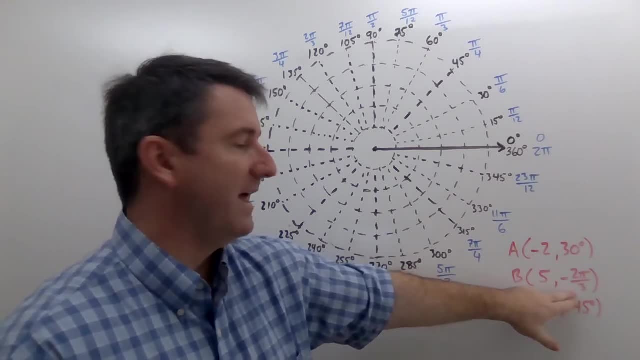 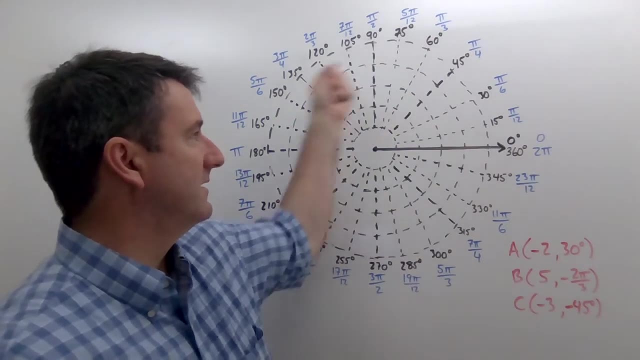 And so all we, if we have a negative value for our angle, for our theta, that just means start here at the polar axis, And instead of going measuring your angle in the clockwise direction, your counterclockwise direction, measure clockwise. 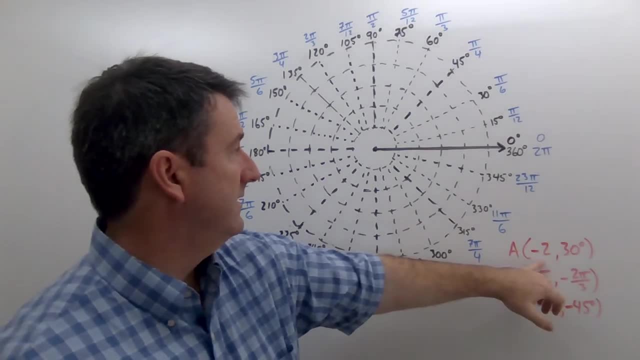 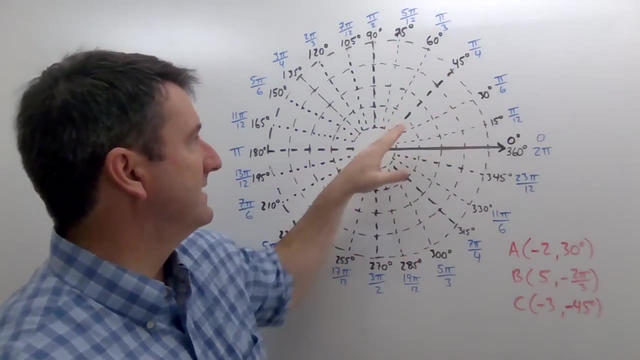 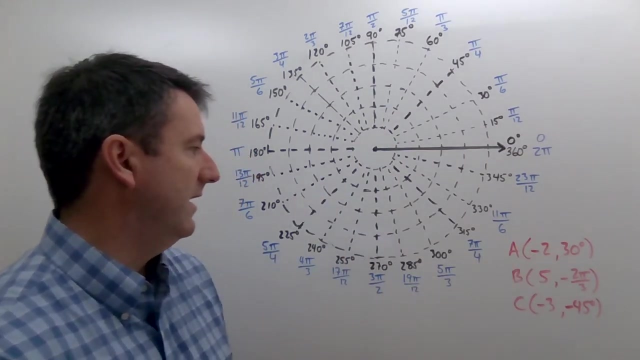 Now for the, for the distance, for the r value. if that's negative, then we're going to go to our angle, and instead of going out toward that angle, we're going to go in the opposite direction. So let's graph these three points and I'll show you what I mean by this. 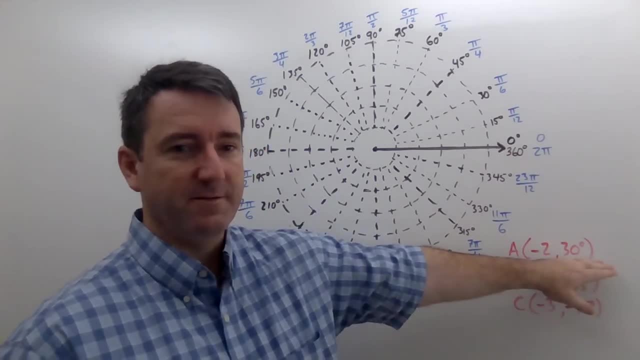 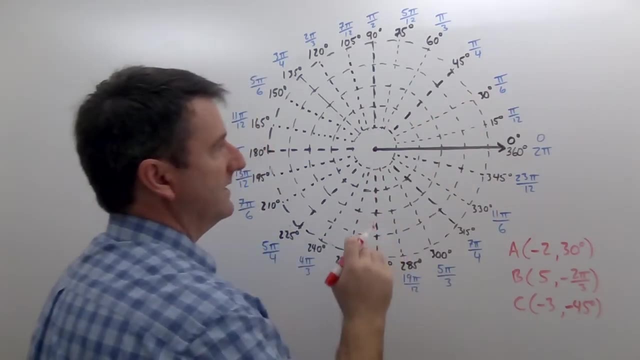 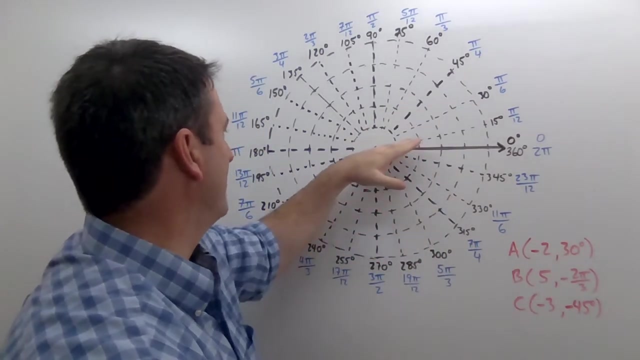 So this first point has a negative r and a positive theta. So we're going to go first to 30 degrees. So it's going to be somewhere out on this, on this line, here out toward 30 degrees, But instead of going out that direction, we're going to go the opposite direction. 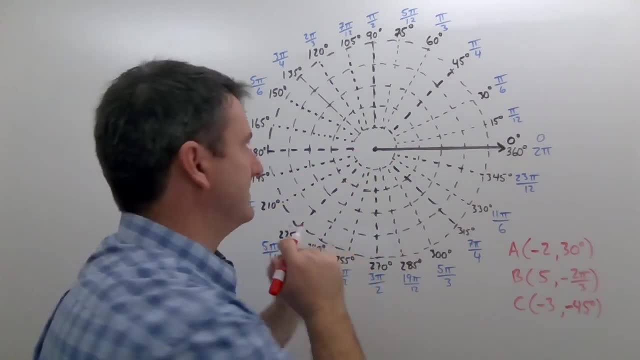 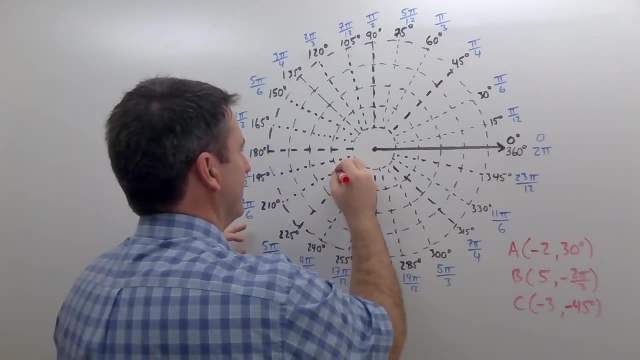 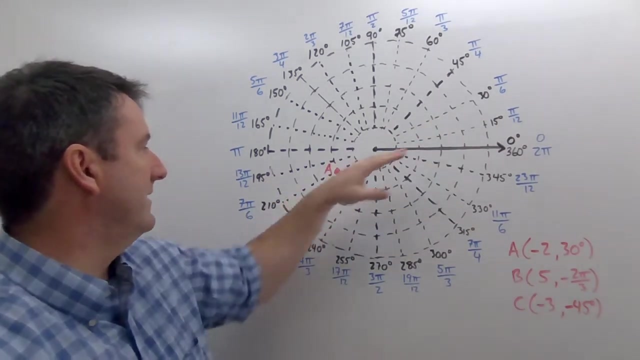 which is going to be out here toward 210 degrees, And we're going to go out two units. so one, two, right, there is going to be the point A, All right, we went to 30 degrees and then went in the opposite direction. two, to give our negative two. 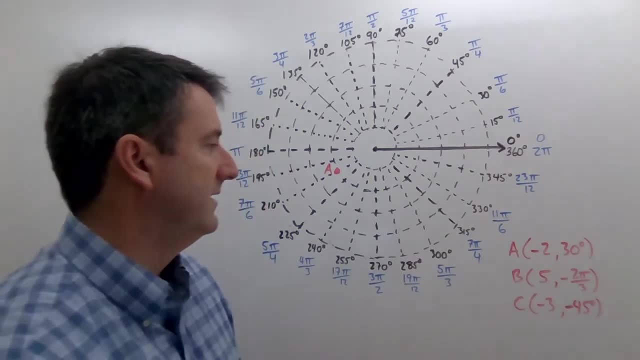 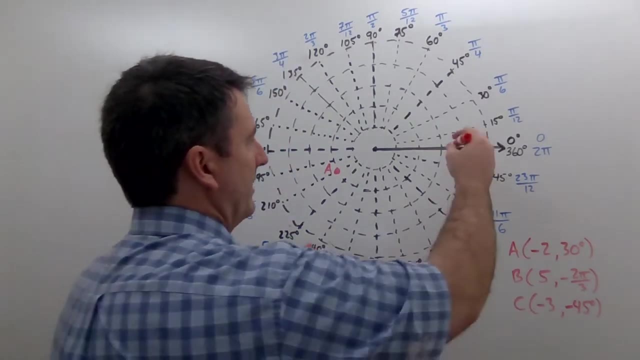 All right. for B we have a positive r but a negative theta. So in measuring negative two pi over three we're going to go this direction: two pi over three. Now we don't have the negative angles labeled on here. 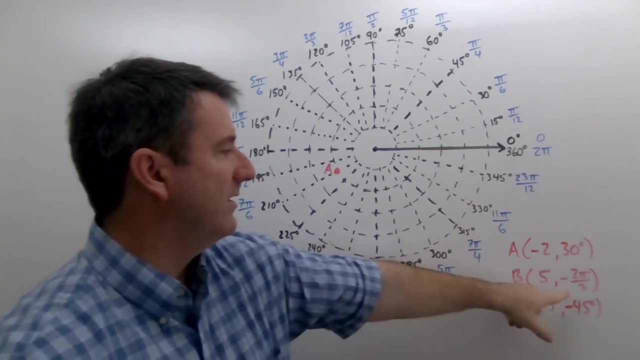 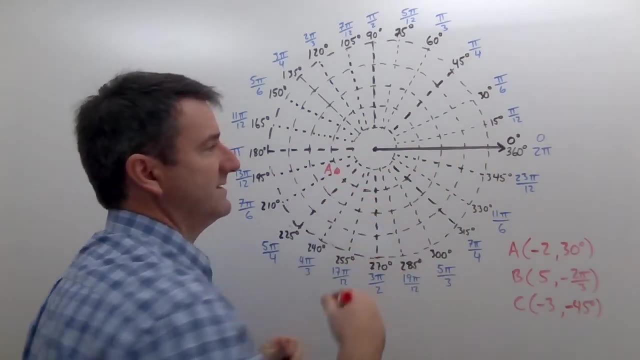 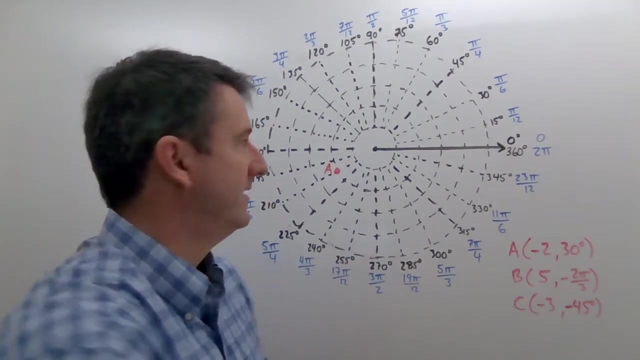 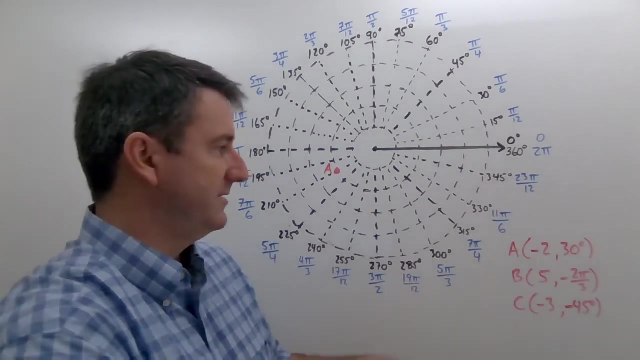 but our angles should always our negative angle. if we add 360 degrees, that's going to tell us what it would be as a positive angle. Or in this case, we add two pi over three, So negative two pi over three. if we add two pi radians, two pi is six pi over three. 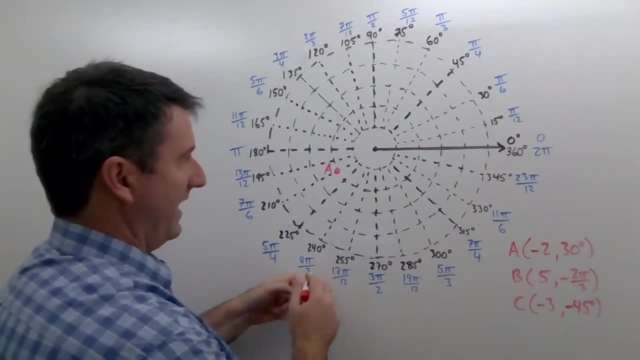 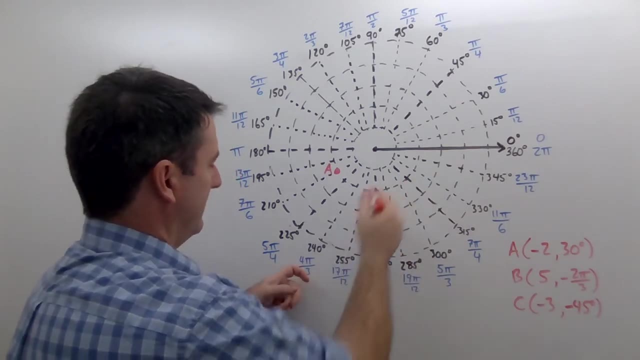 So negative two pi over three is the same as four pi over three. So if we come down here, this right here is the angle: negative two pi over three, coming out here at four pi over three, And we're going to come out five units in this direction. 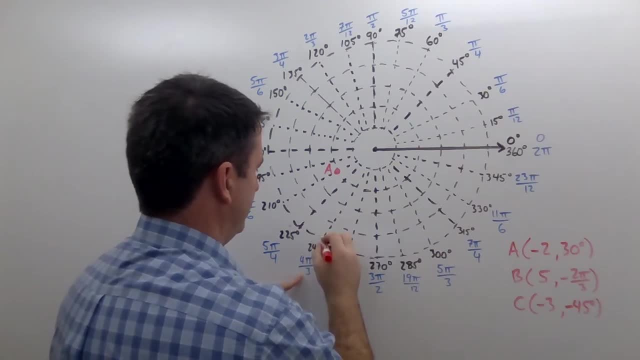 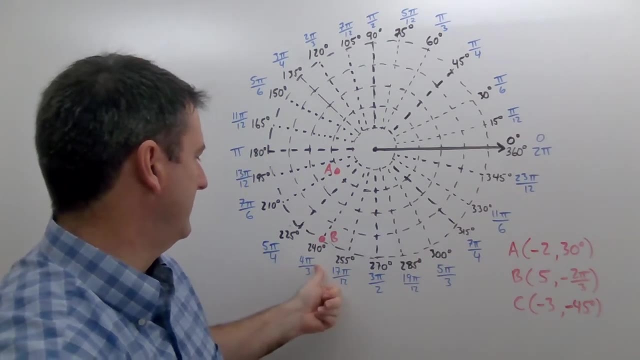 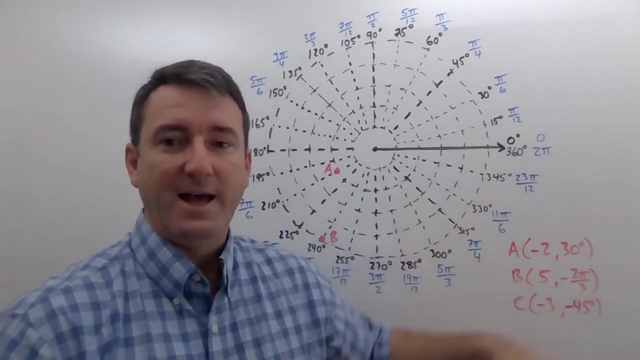 So one, two, three, four, five down here, And that's going to be the point B. So let me make that clear again, to know what the positive version of our negative angle would be. If it's in radians, you're going to add two pi radians. 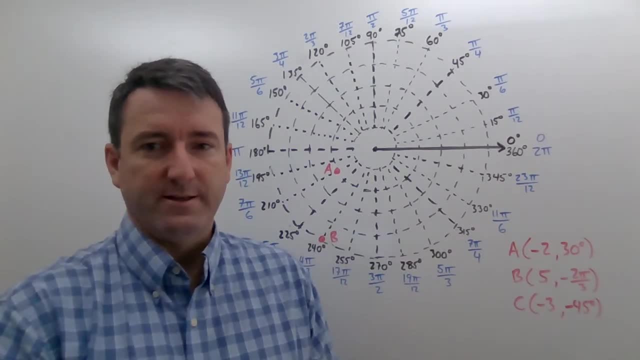 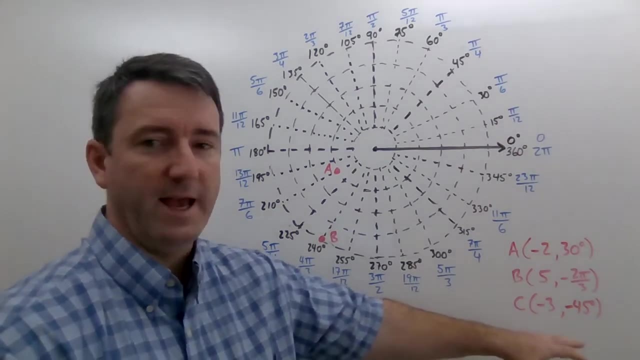 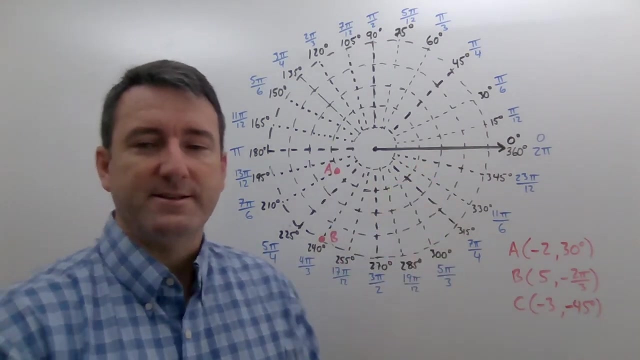 If it's in degrees, you'll add 360 degrees. So let's try that with our last equation. Both of our coordinates are negative, So negative 45 degrees. If we add 360 degrees, that's the same as 315 degrees.